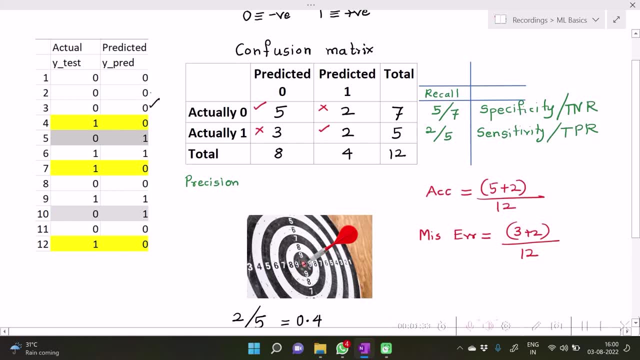 correct predictions are something like this one, this one, this one, three correct predictions, then this one: four correct predictions, five correct predictions. so among eight predicted zeros. so among eight predicted zeros, as, as you see, with this thing we have got five of them correct, so precision for zero can be five upon eight. similar will be the story. 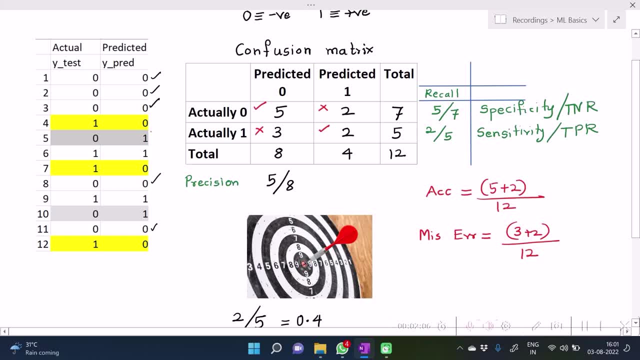 for predicted as one. so as far as ones are predicted, this is the one which is predicted: one, two, three and four. so four ones have been predicted. out of those four ones, this one is correct and this one is correct. other two are wrong. other two are in such a way that here one is predicted, but 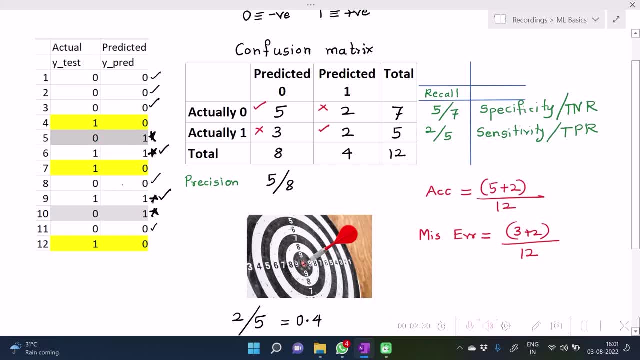 actually it is zero. so this cannot be treated and also this cannot be treated as correct. so hence, the precision is among the four ones, we have got two of them correct. so, as you see that the precision is something which you measure based on the predicted values, and recall is something which you measure based on the actual set of values, 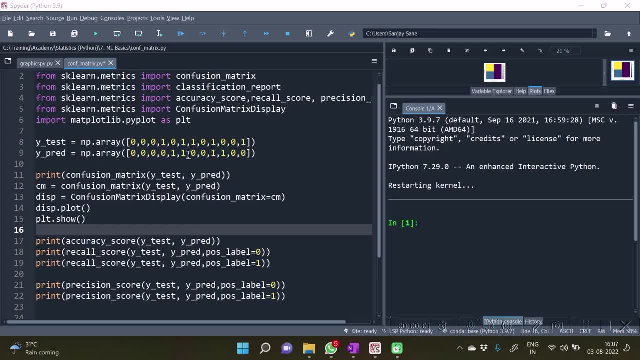 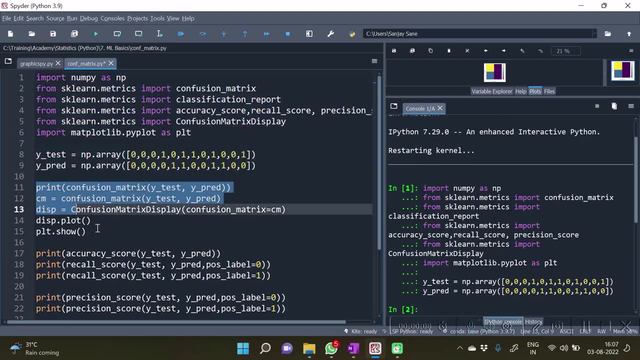 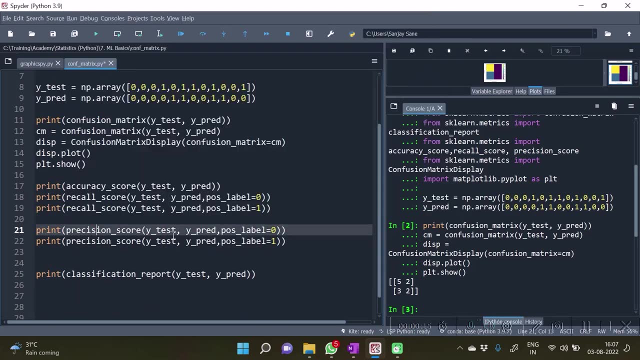 let us see now how we can calculate precision with scikit-learn option. as you see that we have already the confusion matrix here. now it is calculated with the precision matrix and we can calculate the precision matrix with calculated with precision underscore score function. as you see, it is evident from the 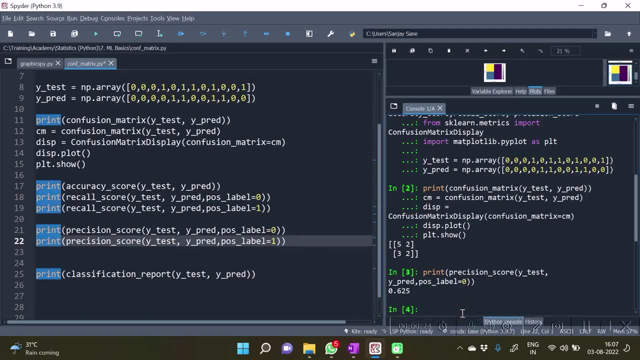 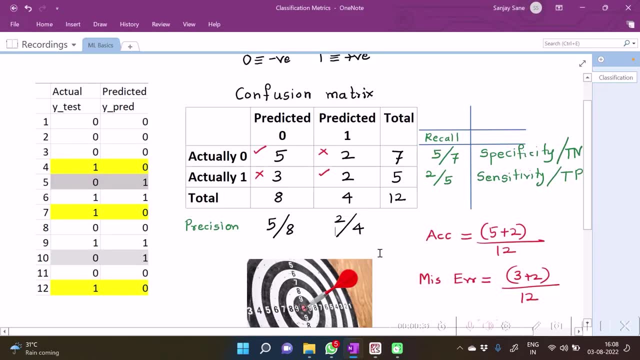 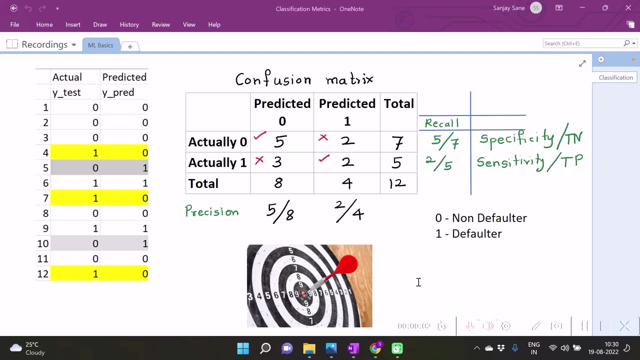 table. it is five by eight for zero. okay, so five by eight, and point six, two, five, and for one it seems to be fifty percent, so to say. ideally, both precision and recall should be one, so to say. ideally, both precision and recall should be one, so to say. ideally, both precision and recall should be one.